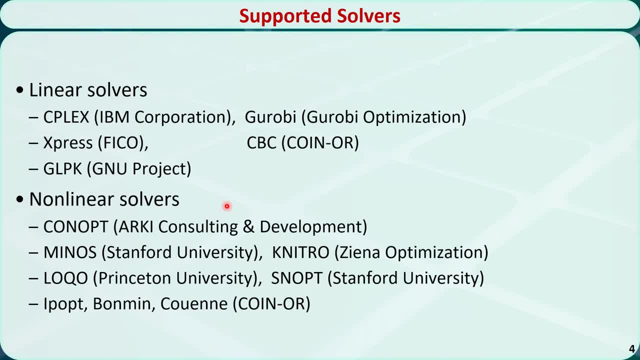 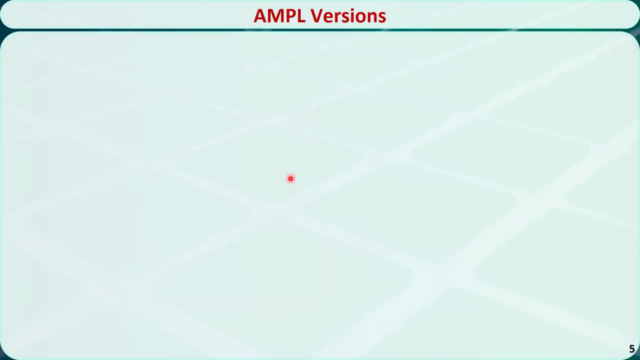 These nonlinear solvers are effective in handling and finding locally optimal solutions to problems involving smooth nonlinear functions using a variety of proven algorithms. AMPL offers four types of licenses for different purposes: 1. AMPL for business targets: large-scale business optimization applications. 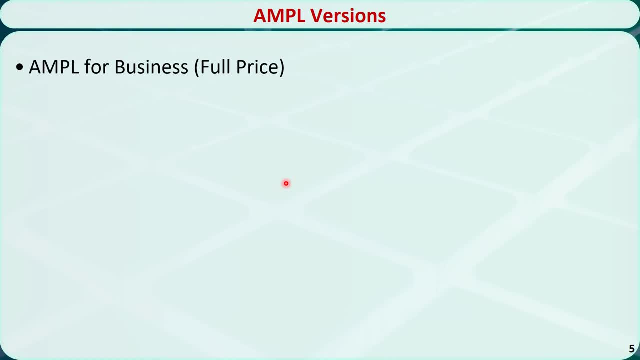 2. AMPL for business targets large-scale business optimization applications. 3. applications in manufacturing, transportation, energy, finance and many other sectors. The license needs to be paid at full price. AMPL for Research targets researchers in universities and corporate labs to solve a diverse range. 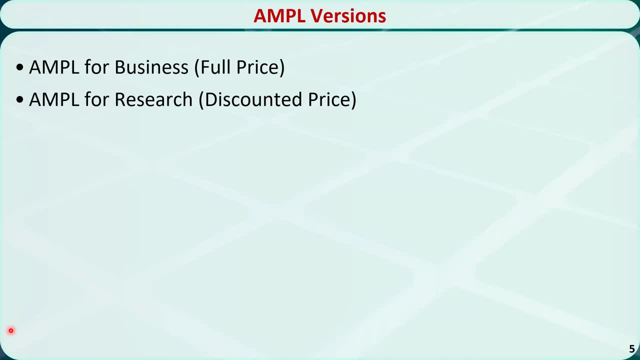 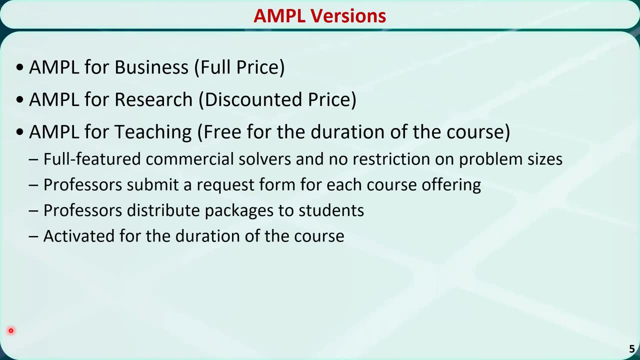 of problems in all fields of engineering, as well as some sciences. The license comes with a highly discounted price. AMPL for Teaching is meant for classroom use to go along with a scheduled course throughout a semester. It is completely free and comes with full-featured commercial servers and no restriction on problem. 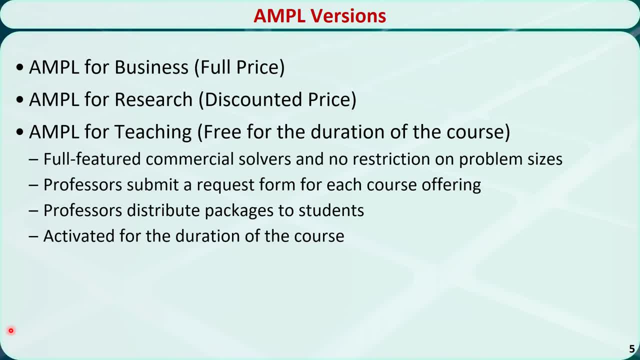 sizes. Professors submit a request for the course. then they will receive a special version of the software. They can freely distribute it to the students so they can install on their own computers. The students can use it for the duration of the course. 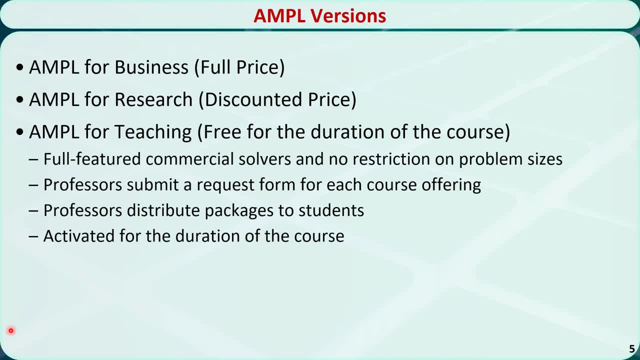 It will stop working after the course ends. AMPL for Students is a free demo. It is a demo version that is aimed to help students quickly get familiar with formulating and solving small-scale optimization models. There are some problem size restrictions. For linear programming problems it is limited to 500 variables and constraints. 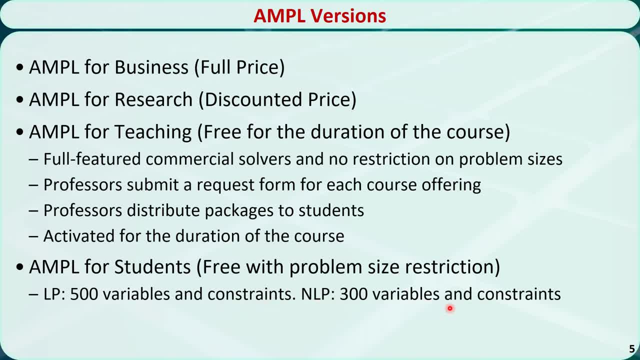 For nonlinear programming problems, it is limited to 300 variables and constraints. We can also use the NEOS server, which contains many free online solvers. The limitation is that the programming is limited. Problems submitted will be put in a queue. If the server is busy, it may take a while before your problem is processed. 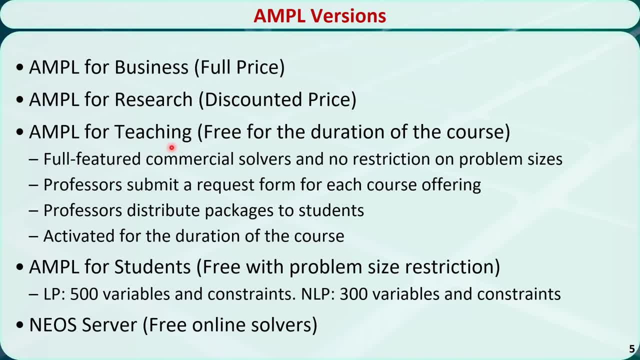 I have previously used the AMPL for Teaching version in my class and distributed it to my students. Later I found out that the free AMPL for Students version was adequate for illustrative purposes when teaching students the basic concepts of operations research, because we were only dealing with small-scale problems in the course. 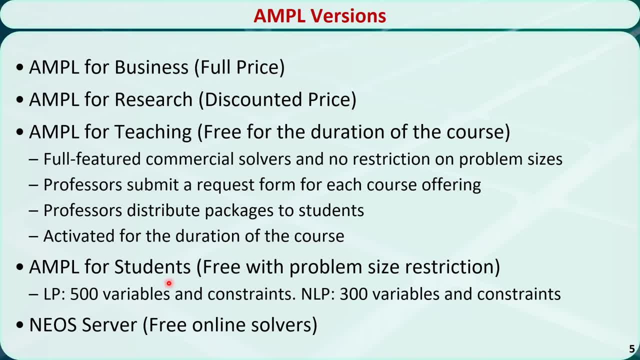 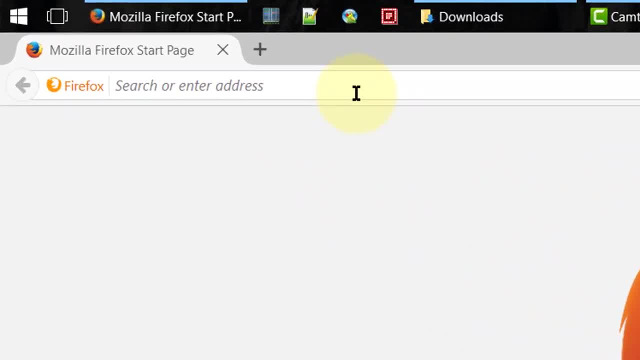 Therefore, I will talk about the AMPL for Students version in the next video. Thank you, Bye. We will learn about how to download and install this AMPL for Students version For a Windows computer. you need to go to this website: amplcom. 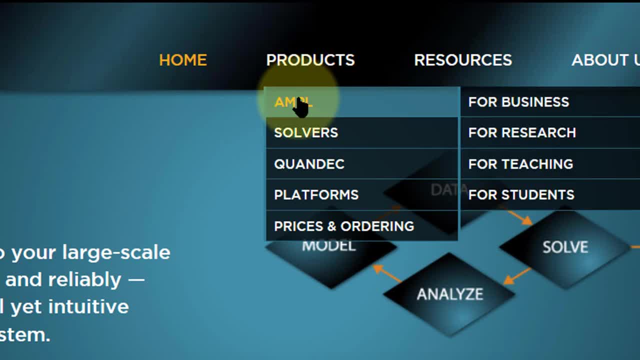 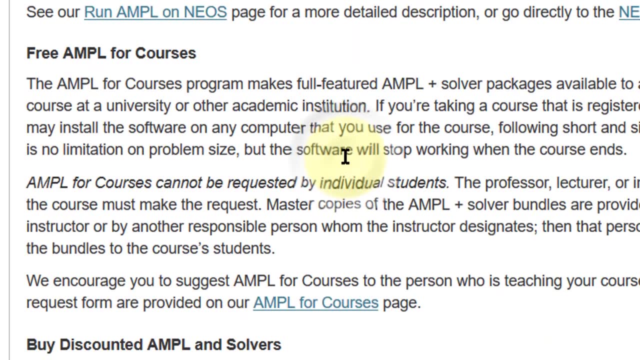 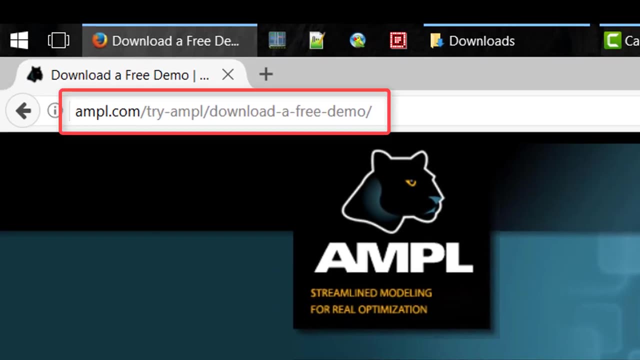 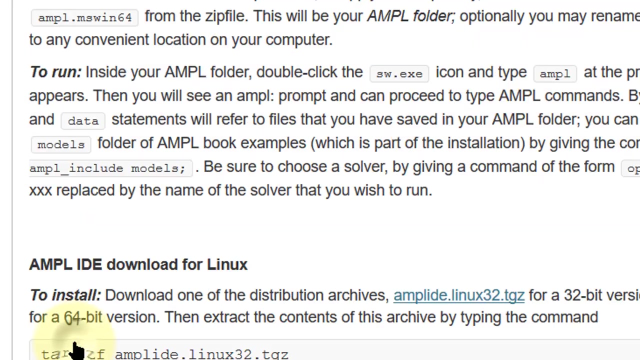 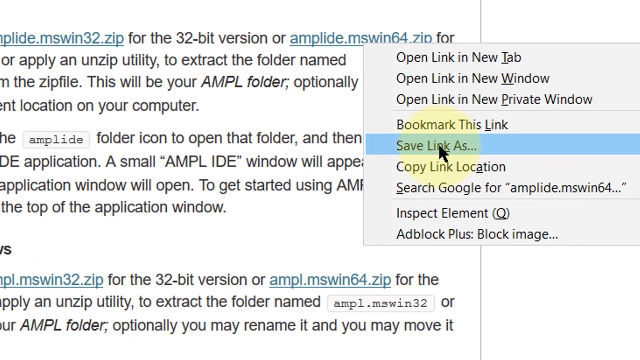 Enter the menu Products, Ampl, Select For Students, Then click Demo version. Download a free demo. Alternatively, You can directly go to this website amplecom. try ample. download a free demo. Now click Windows and download this compressed ampleidemswin64.zip file. 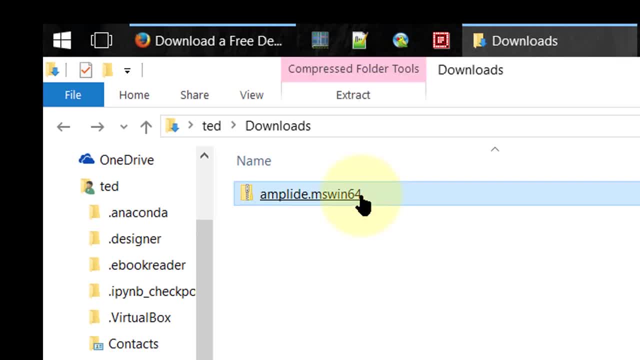 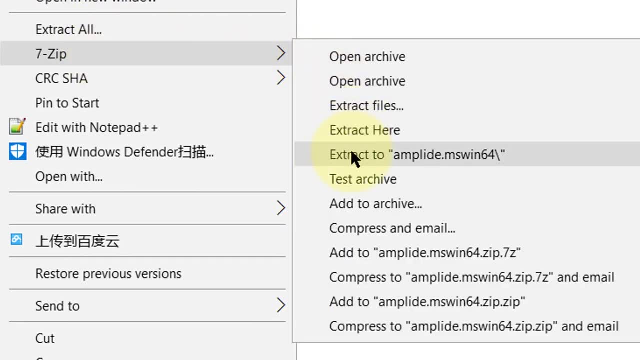 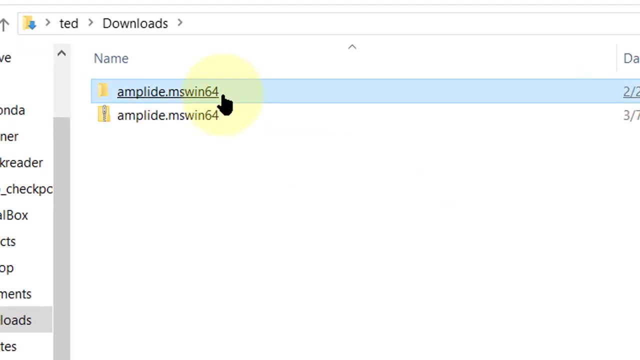 It is about 160 MB. The installation is really easy. You just need to unzip the file to extract the folder named ampleidemswin64.. You may rename it and move it to another location on your computer. To run ampleide you need to get inside the folder. 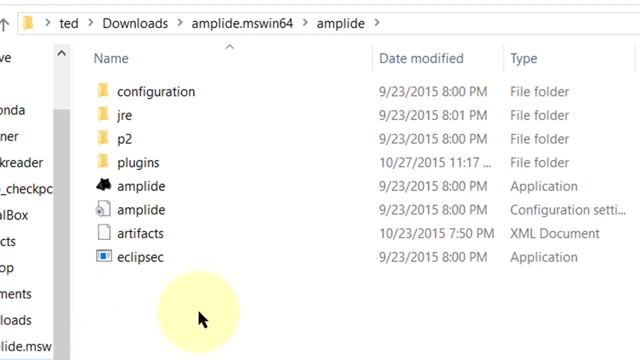 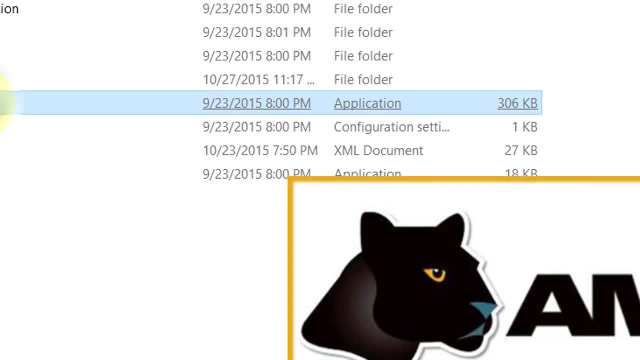 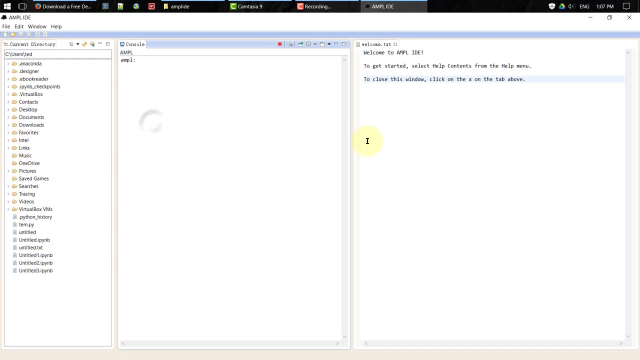 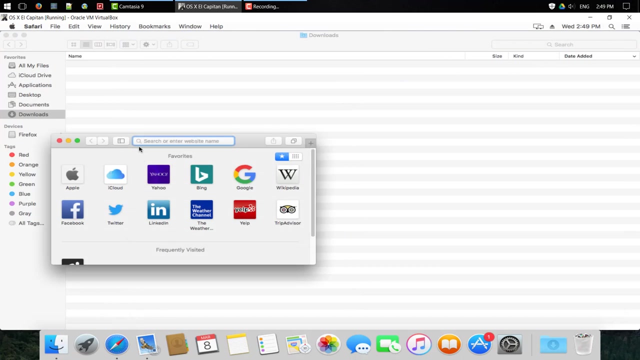 Double-click to open the ampleide folder and then double-click the ampleideexe file. It will bring you to the ampleide folder. Open the ampleide window For Mac computer. the only difference is the last step. You need to go to the website amplecom. 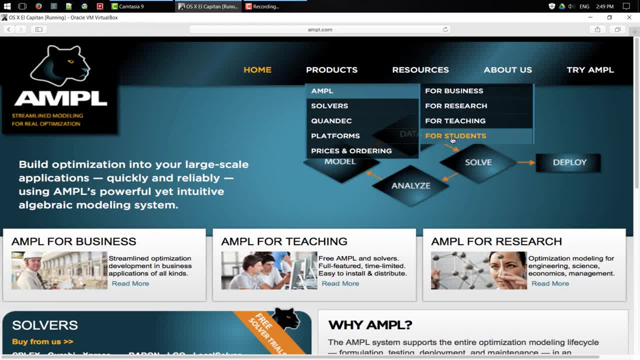 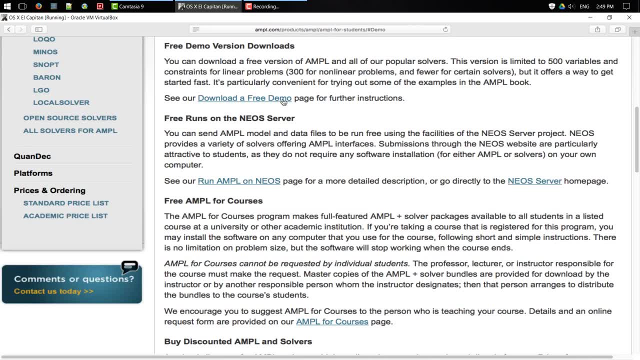 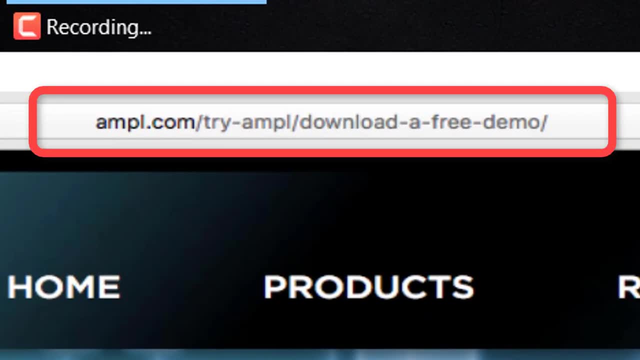 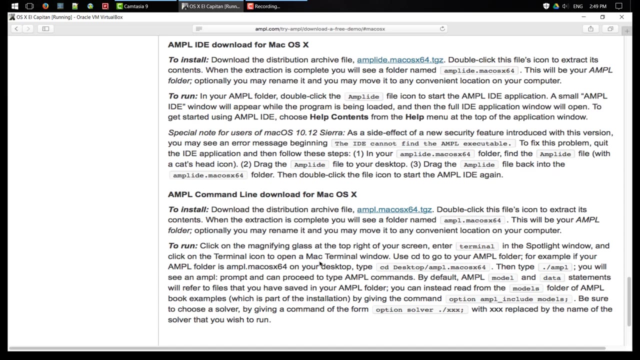 Enter the manual products: ample, select for students, Then click demo version. Download a free demo. You can also directly go to this website, amplecom. try ample. download a free demo. Click macOS instead of Windows and download this compressed ampleidemacos64.tgz file. 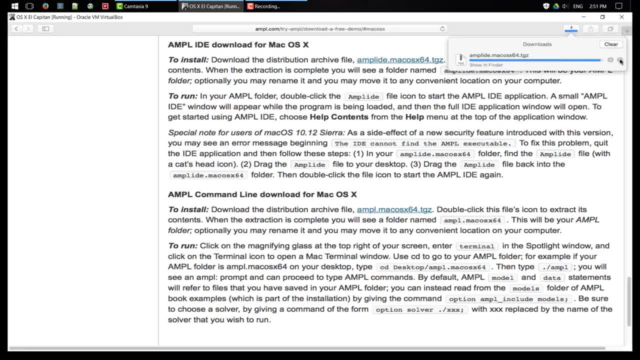 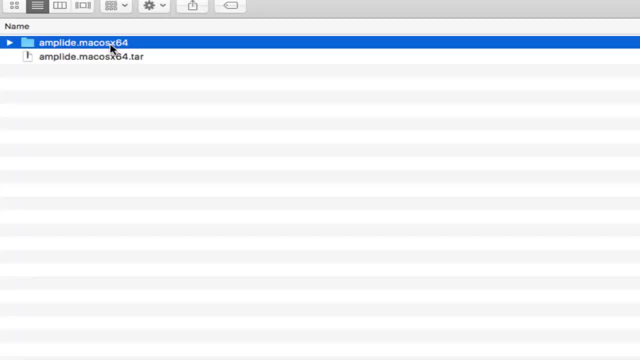 To install. you just need to double-click the tgz file to extract the folder named ampleidemswin64.zip. You can also directly go to this website: amplecom. Try ample. You may rename it and move it to another location on your computer.